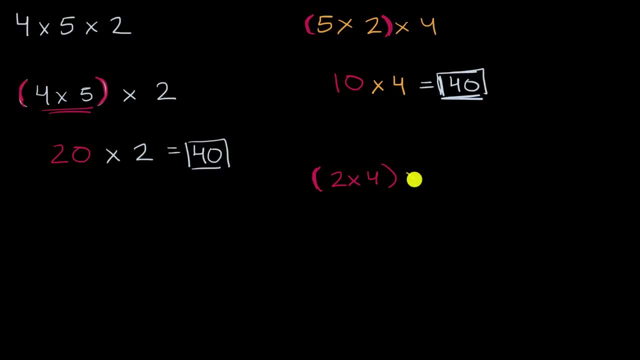 Two times four and then multiply that by five. What is this going to be equal to? Well, you might notice again: this is two times four is eight. You multiply that times five. Well, once again we got 40.. 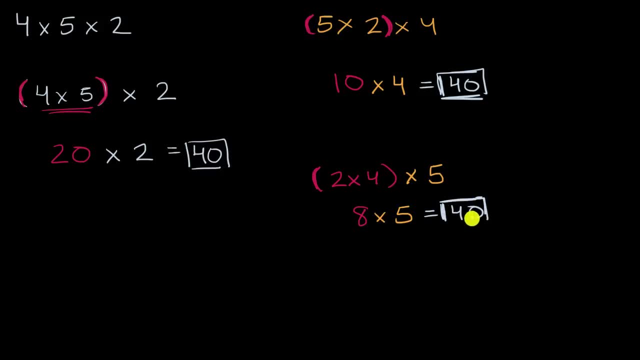 So you might see a pattern here. It doesn't matter which order we multiply these things in. In fact you could write four times five times two, You could do the four times five first, four times five times two, Or you could do four times five times two. 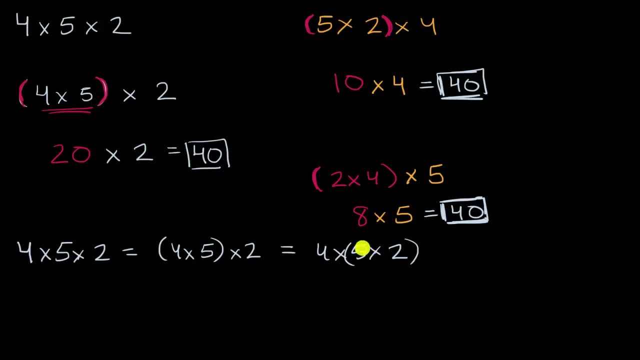 So you could do four times five times two. So it doesn't matter which order you multiply these things in, In every case you are going to get 40.. Now there's a very fancy term for this: the associative property of multiplication. 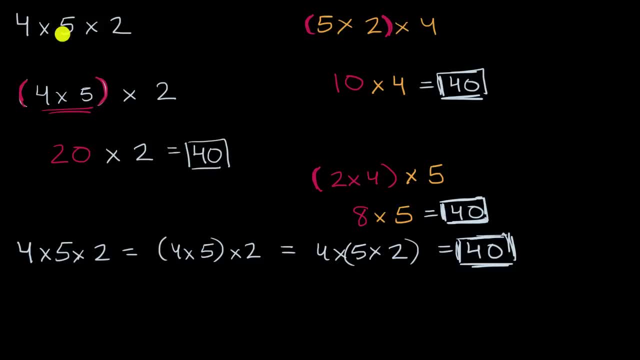 But the main realization is- and it's not just true- with three numbers. In fact, you've seen something similar with, say, two numbers, where it doesn't matter what order you multiply them in, But what you see is with three numbers. 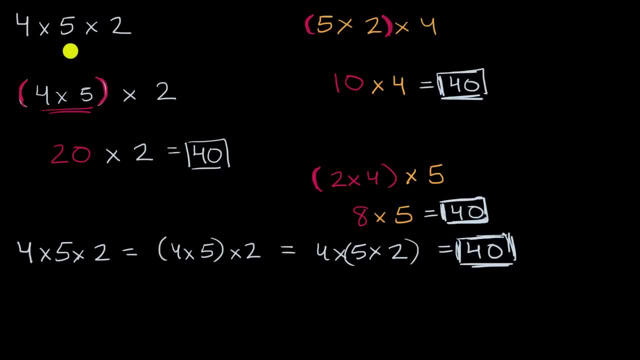 and even if you tried it with four or five or really a thousand numbers being multiplied together, as long as you're just multiplying them all, it doesn't matter what order you're doing it with, It doesn't matter in what order you associate them with. 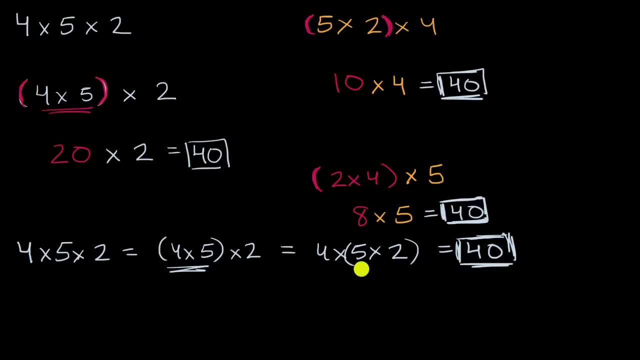 Here we did four times five first. four times five first. Here we did five times two first. But in either case we got the same result. And I encourage you, after this video, try to draw it out, Try to think about why that actually makes. 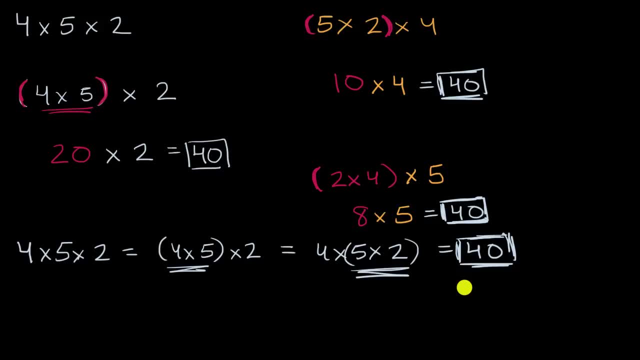 a very intuitive sense why this is true in the world. And it's nice because it simplifies our life when we're doing mathematics, not only now, but in our future mathematical career. 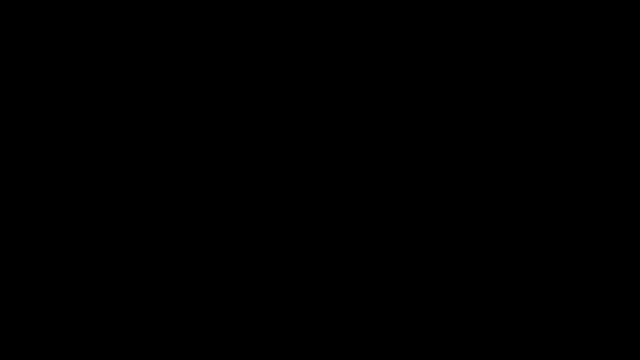 It doesn't take long to realize that taking higher and higher powers of binomials can get painful. But let's just work through a few just to realize how quickly they get painful. So if we take the binomial a plus b, it's a binomial because it has two terms right over here.